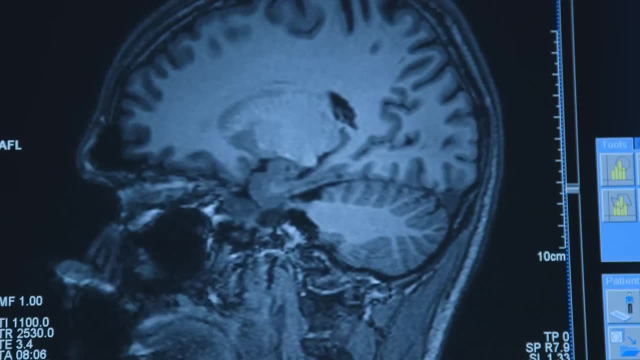 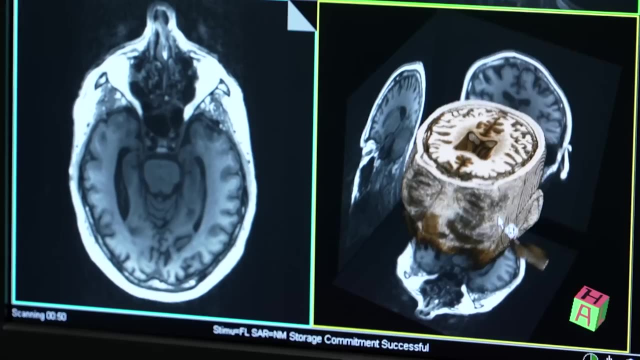 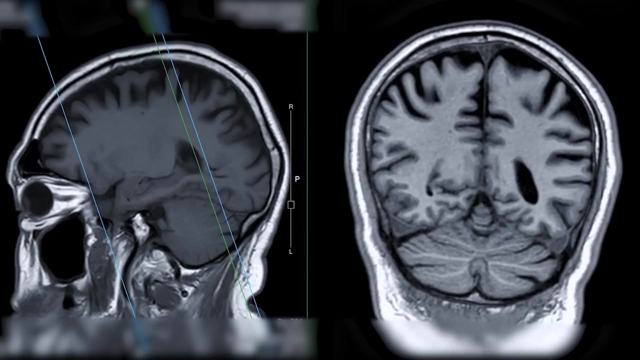 to the safe millimetre resolution of MRIs capable of creating a 3D reconstruction of the body rather than a flat 2D image, Achieving all of that without any moving parts. Imaging in medicine relies on collecting signals from the body based on the innate physical. 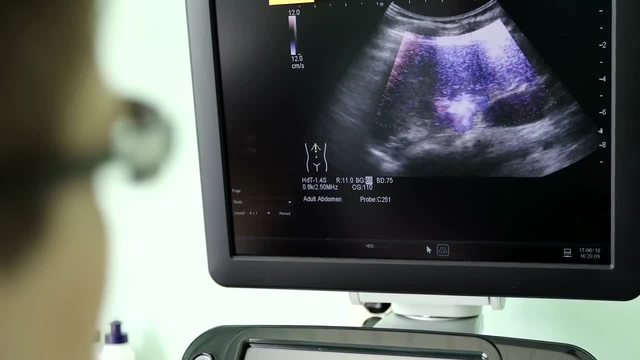 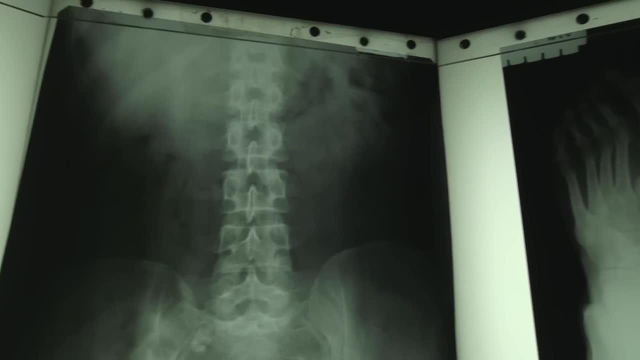 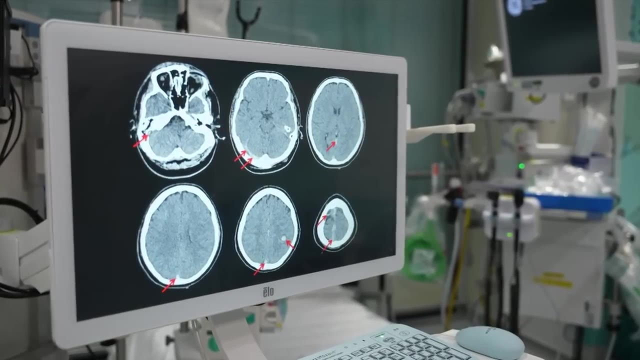 properties of tissues. Ultrasound imaging relies on how sound waves bounce off of the tissues of different densities. X-rays form images based on the absorption of high energy radio frequency waves. Magnetic resonance imaging, however, relies on something far less intuitive: the quantum properties of the hydrogen atom. 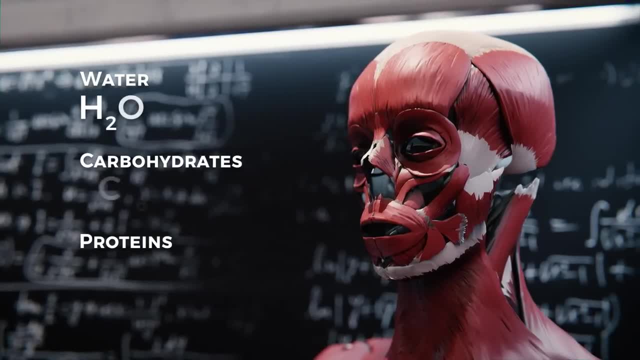 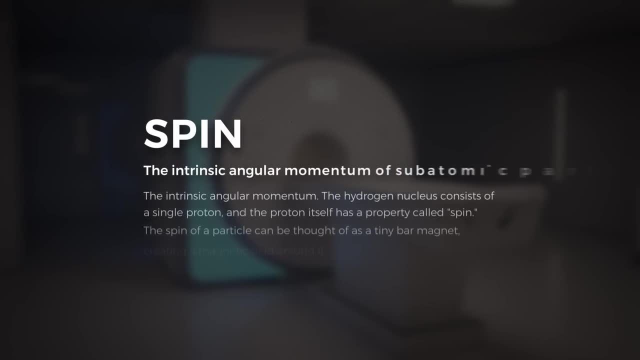 The human body is teeming with hydrogen atoms located in water, carbohydrates and proteins. To image the body, MRI machines exploit a quantum property of these hydrogen atoms, a property called spin. How it does this is a marvel of modern science: The human body. 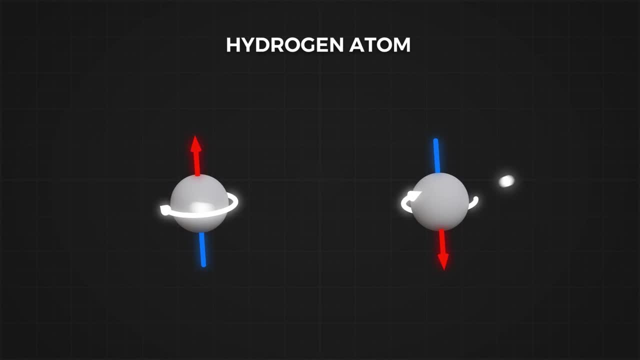 has modern physics and engineering. Spin is an innate property of particles, just like mass and charge. Spin makes particles behave like tiny bar magnets. The proton inside the hydrogen nucleus behaves like a magnet. The orientation of its magnetic north is described probabilistically. Under normal circumstances, this probability is evenly distributed. This: 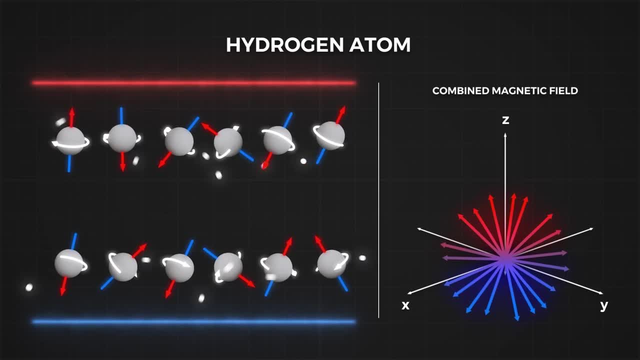 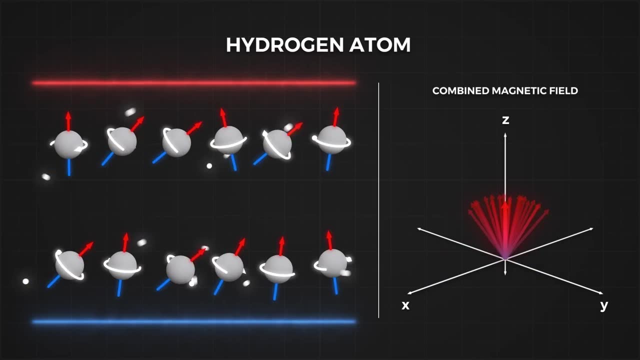 means the combined magnetic field of many hydrogen atoms cancels out. But this change is when the hydrogens are inserted into a large external magnetic field, just like the ones MRIs create. This changes the distribution of the tiny magnets, augmenting the number. 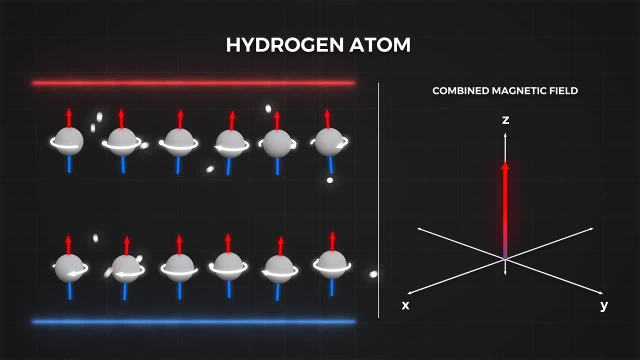 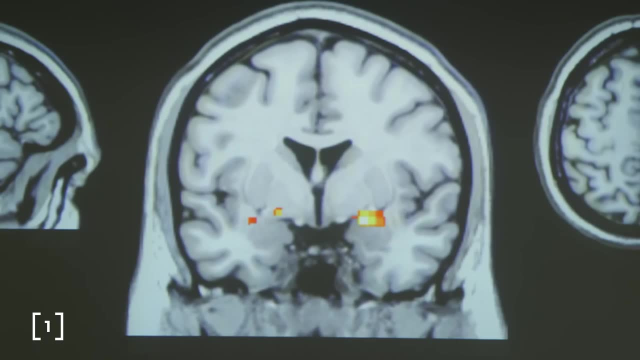 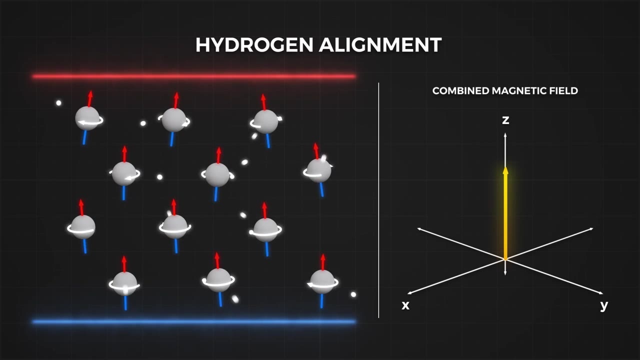 of atoms aligned with the external magnetic field. This imbalance is the source of the MRI signal. We can manipulate these tiny magnets to produce signals that can be processed into images. Once the atoms are aligned in the machine's incredibly strong magnetic field, the machine gives them a tiny nudge using a magnetic radio frequency pulse. This pulse 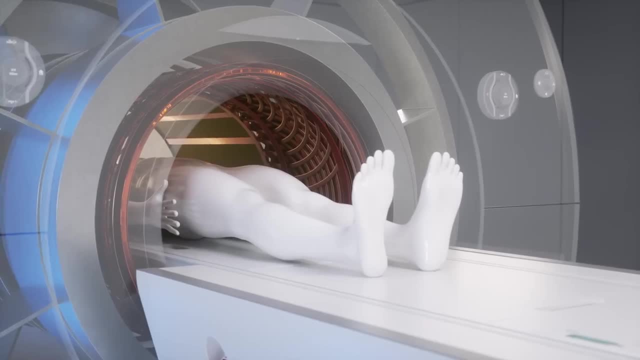 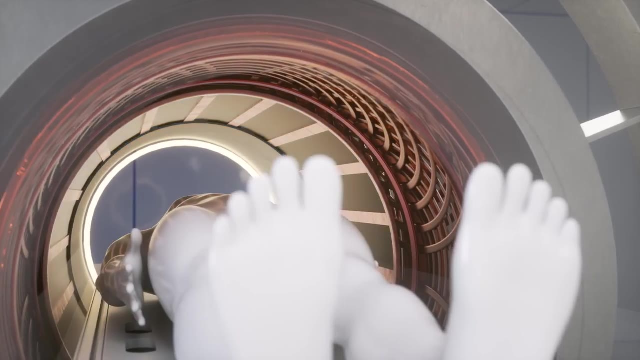 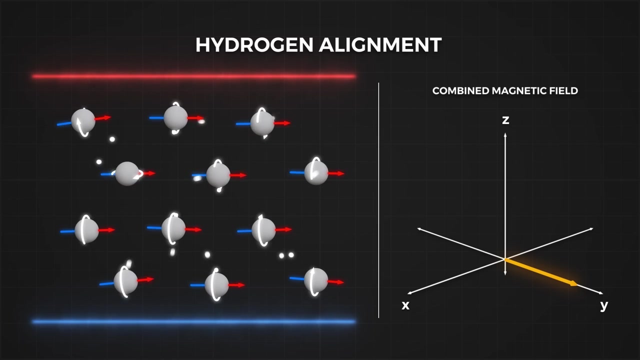 comes from this set of coils inside the machine that sends pulses by simply applying an alternating current through its coils at a very specific frequency. This nudge misaligns these hydrogen bar magnets to shift their magnetic field perpendicularly to the large magnetic field the machine is creating. Naturally, the spins want to align their orientation back to their 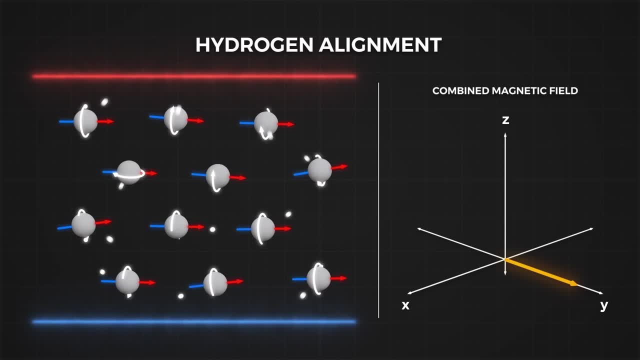 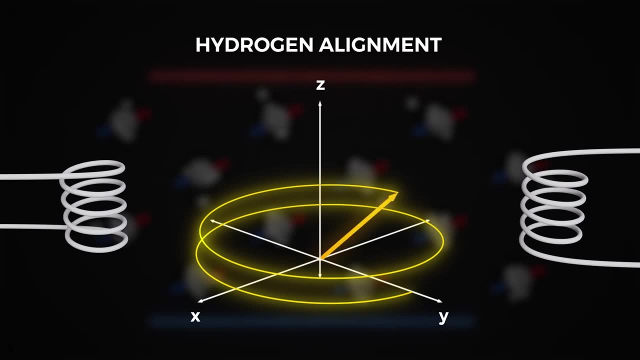 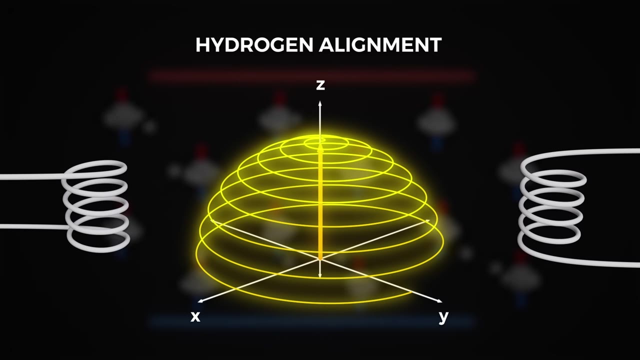 original position, Aligning with the machine's magnetic field, But they don't fall back immediately. they decay in a spiralling motion. This decay causes a changing magnetic field and by placing a coil of wire nearby, this changing magnetic field can induce currents that can be read. 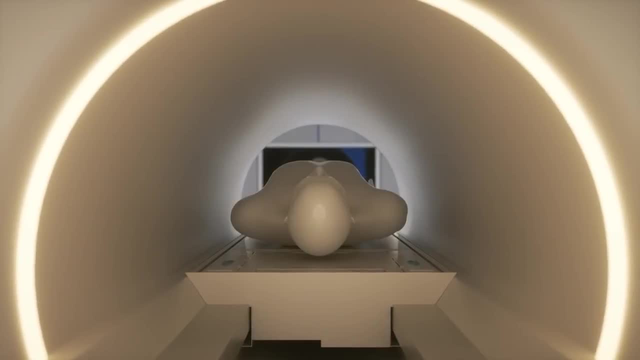 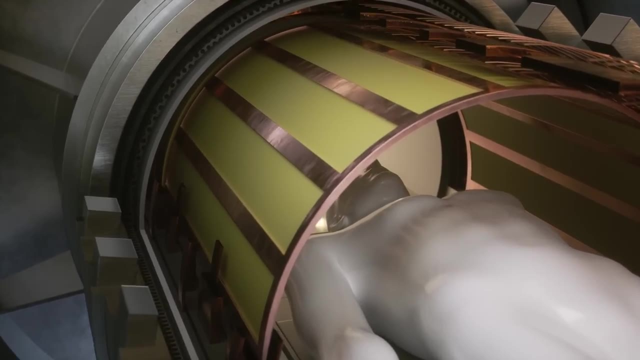 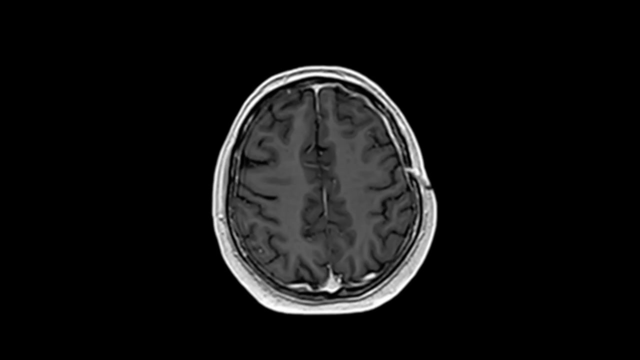 as a clear signal. MRI machines can use the same coils to send the nudge pulses and to read the signal from the body. These coils are placed here as close to the patient as possible, but still inside the MRI tube For higher contrast and resolution. some machines use separate. 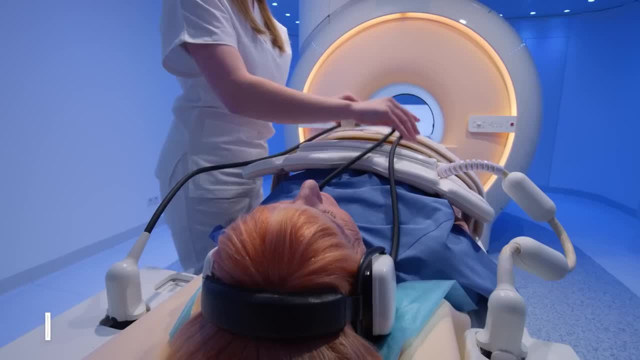 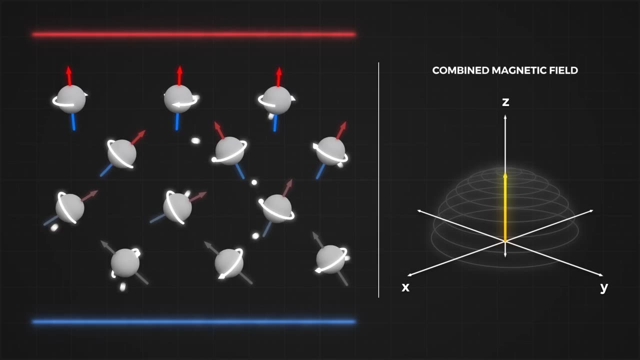 coils to transmit pulses and to receive the signal. This allows the receiver coils like these to be placed much closer to the body, maximising the strength of the signal. We can increase the number of hydrogens aligning with the external magnetic field by increasing 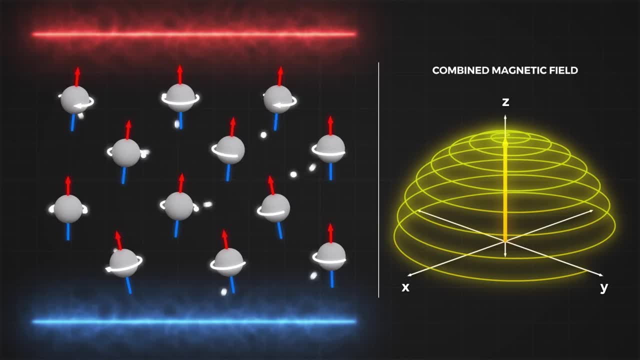 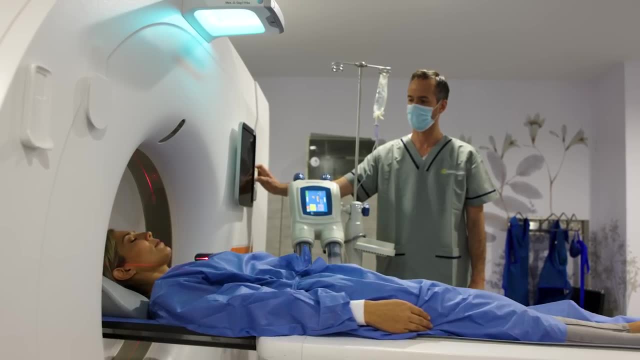 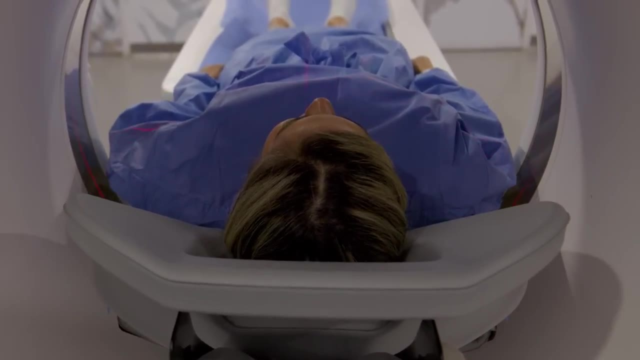 the strength of the external magnetic field. In turn, the hydrogen magnet can induce a larger current as it spirals back. So by simply increasing the strength of the MRI's field we increase the strength of the signal collected and therefore improve the image quality. 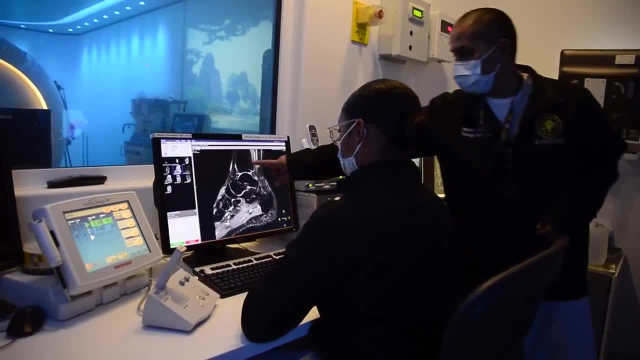 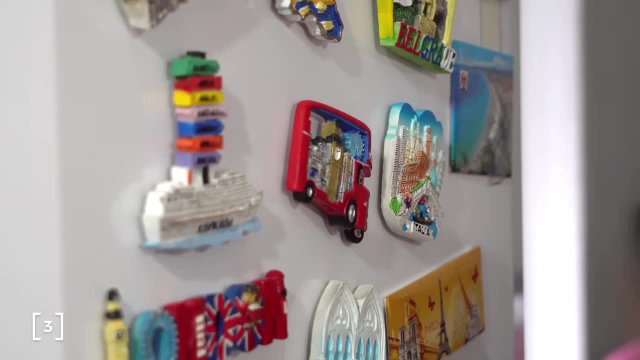 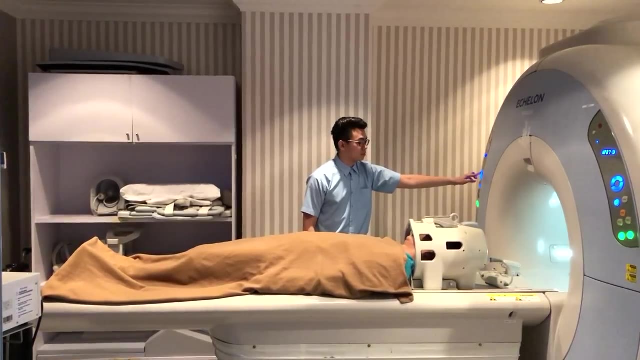 Common MRI field strengths are 1.5 to 3 Tesla. Around 300,000 times stronger than the earth's magnetic field and 30,000 times stronger than your common fridge magnet. You absolutely do not want anything ferrous around these machines during operation. A field this strong. 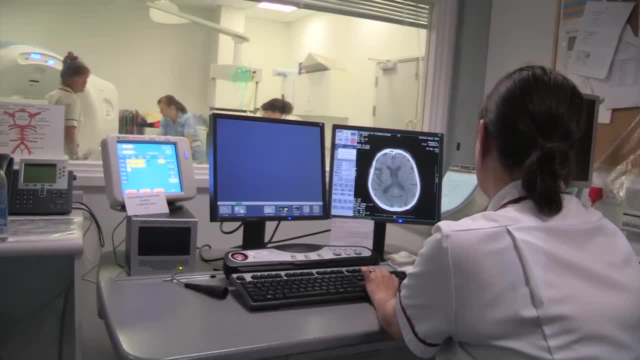 can lift nearby wheelchairs straight off. How often does a magnetic field need to be set up? The magnetic field is set up by the the ground For research purposes. MRIs can produce even higher magnetic fields, up to 20 teslas. 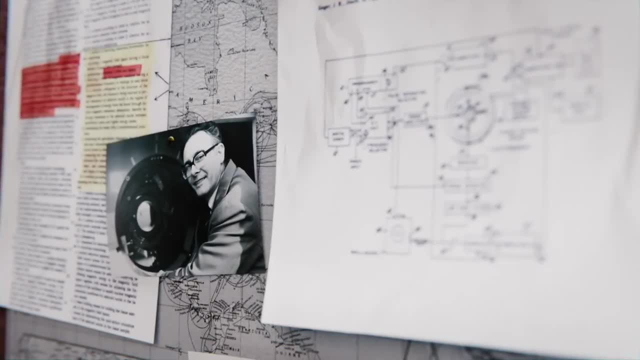 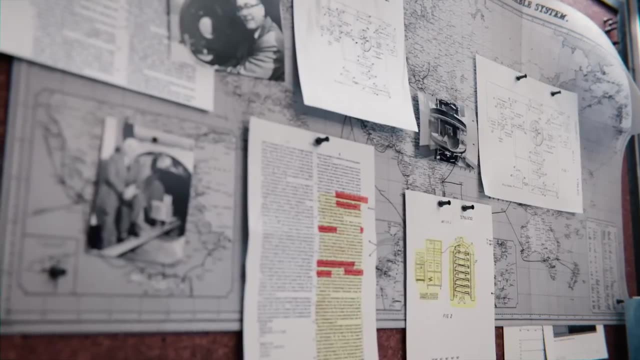 Achieving this intense magnetic field comes as no easy feat. Early MRIs used permanent magnets as their source of the main magnetic field, but only reached strengths of 0.5 tesla, limiting the resolution of the machines. Electromagnets can be used to reach stronger. 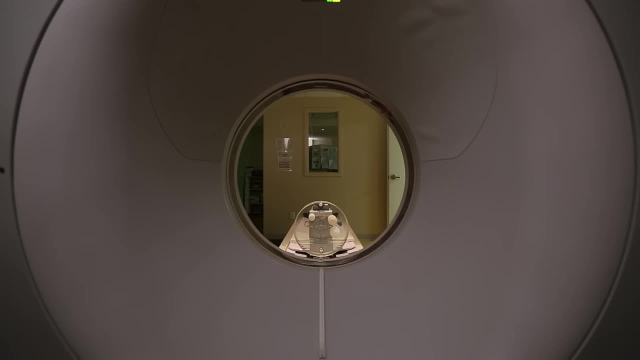 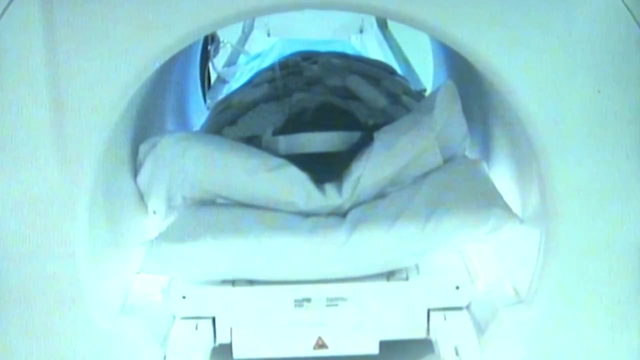 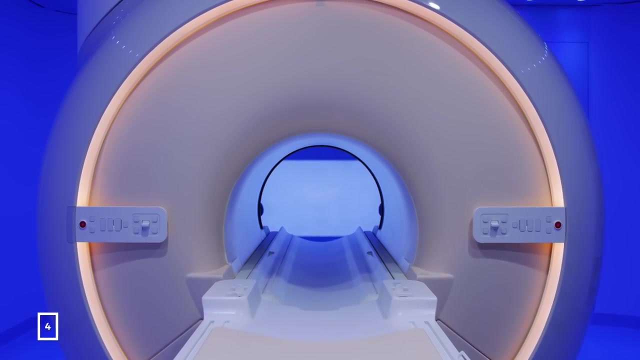 magnetic fields, but standard electromagnets can't produce a 1.5 tesla field. Higher magnetic fields require higher electric currents that would melt ordinary wires. To achieve larger currents in the wires, engineers required superconducting coils. Superconductors are another sci-fi. 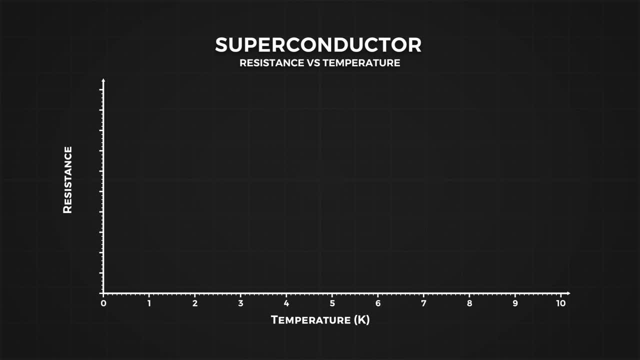 technology. Temperature affects all metallic conductors, with resistance gradually lowering with temperature, But superconducting materials are special in that they're really the only materials that can produce superconducting coils. Superconductors are the only materials that can produce superconducting coils. The resistance drops to zero at temperatures. 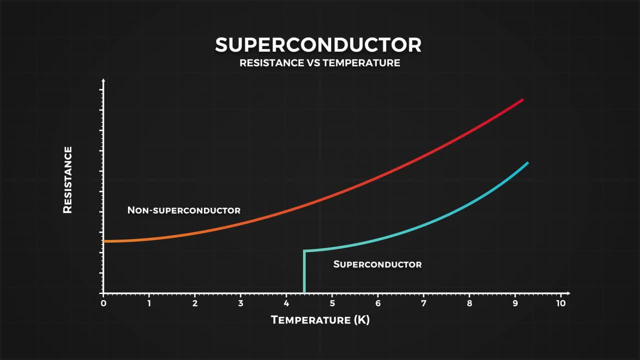 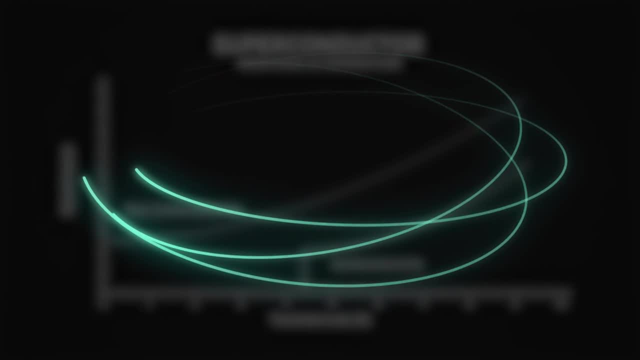 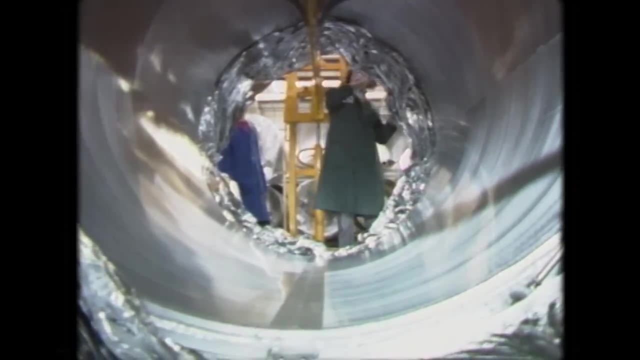 close to minus 273 degrees Celsius or absolute zero. In theory, when this happens, an electric current could travel in a loop of superconducting material indefinitely, never needing a power source. In reality, this means that the main superconducting coil in MRIs does not consume any. power directly. Rather, the main consumption of energy is just to keep the coil cooled down, so the current will travel endlessly, leaving the MRI magnet permanently on. The energy needed to run an MRI for a full year is equivalent to 25- 4 person households- around 130,000 to 140,000 kWh per year. 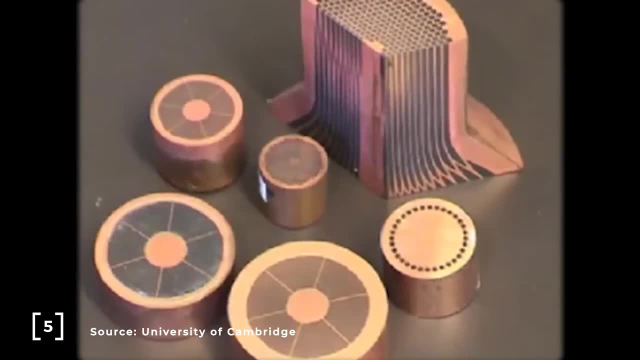 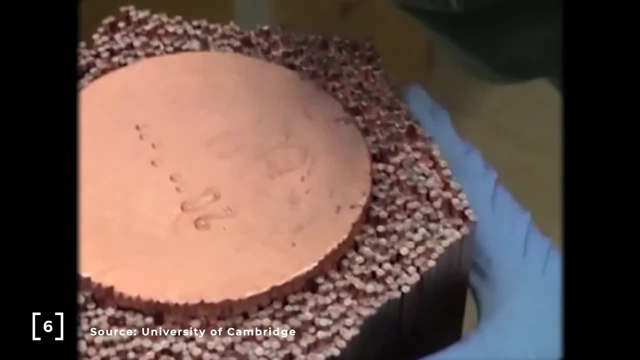 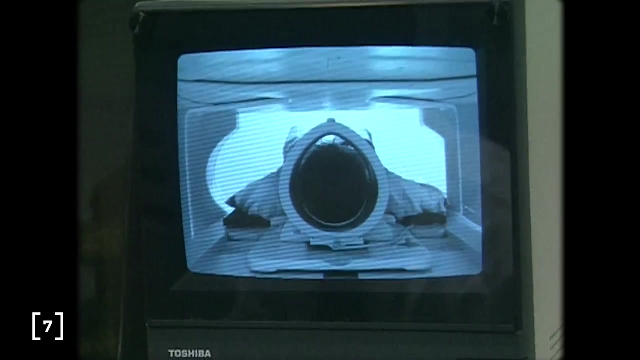 The most common superconducting material in MRIs is niobium titanium. The demand for high resolution images is so large that 80% of all the niobium titanium we extract from the earth goes into MRI machines To achieve the incredibly low temperatures needed for superconductivity. 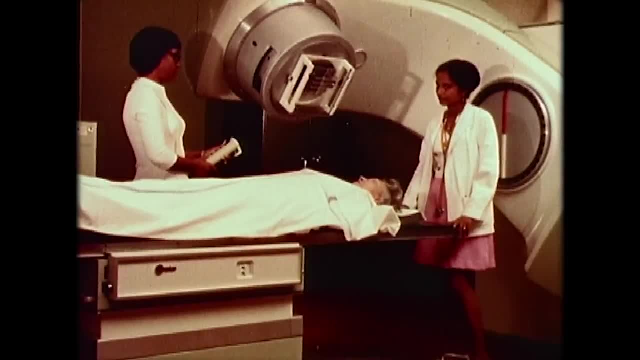 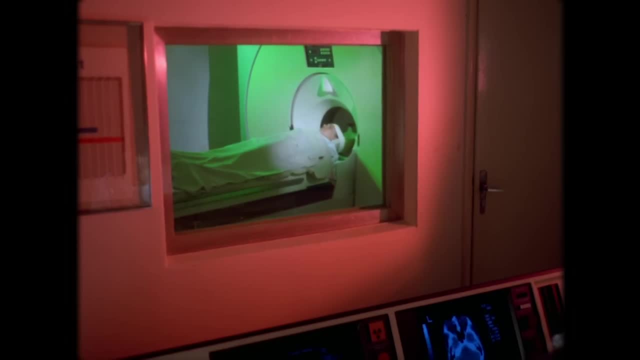 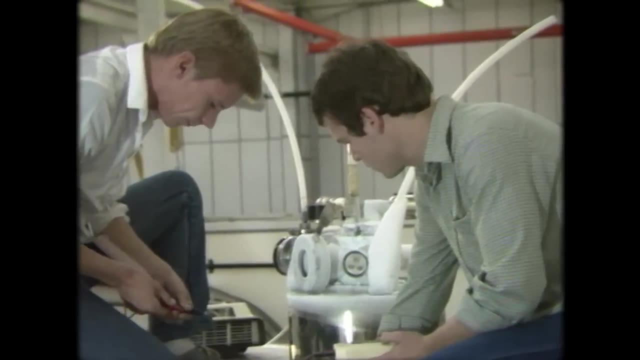 we need a very cold refrigerant. Early MRI machines used to submerge their superconducting wires in a bath of liquid helium. pouring 1000 litres of liquid helium at minus 269 degrees Celsius into the machine to cool the superconducting coil as close to 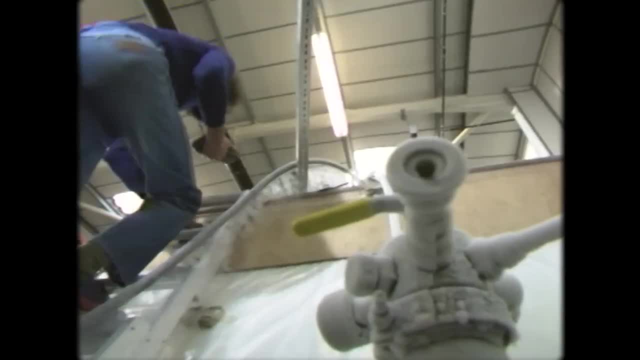 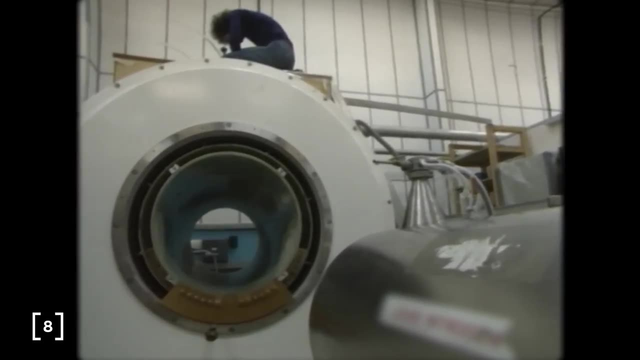 absolute zero as possible. This evaporated the helium, allowing it to escape the machine as a gas. Meaning early MRI machines required regular refillings of liquid helium. Even though helium is an incredibly common gas in the universe, it is so light that it can escape. 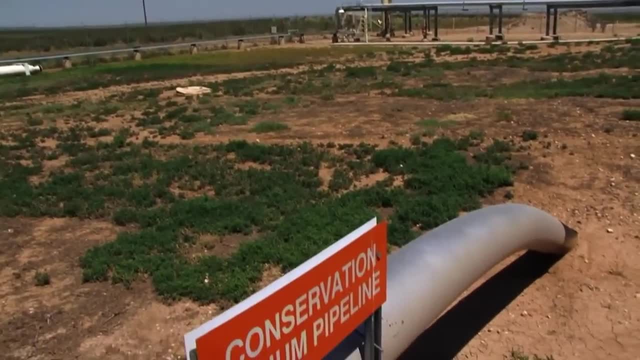 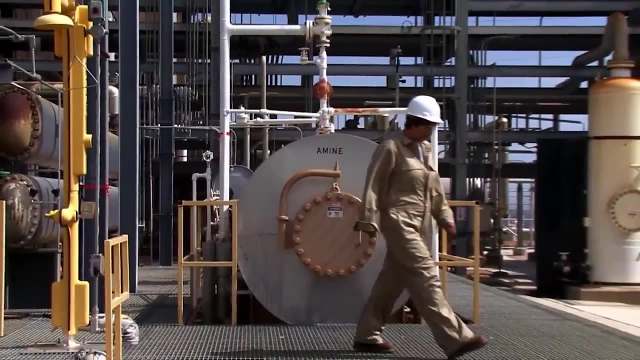 our atmosphere into space. We extract helium from underground gas caverns, where it accumulated as a by-product of uranium and thorium radioactive decay. But once we allow the helium to escape into the atmosphere, it is gone for good, floating to the top of our atmosphere and gradually being 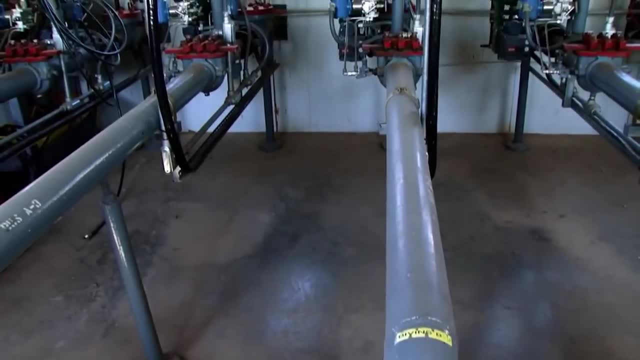 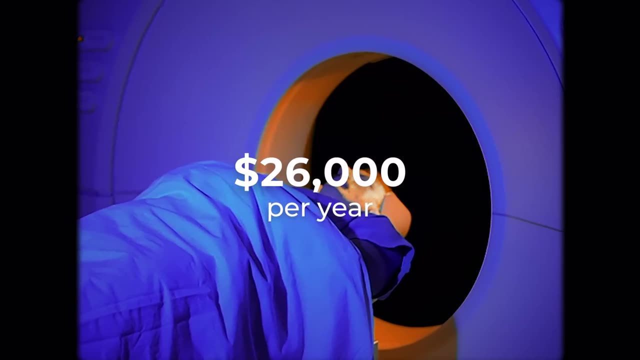 blown into space as a gas. This is the most common superconducting material in the universe. We will eventually run out of natural helium. This method of cooling was costly and unsustainable, costing up to $26,000 per year in helium refills. 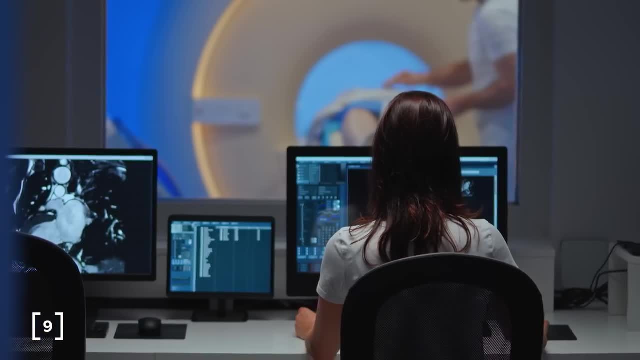 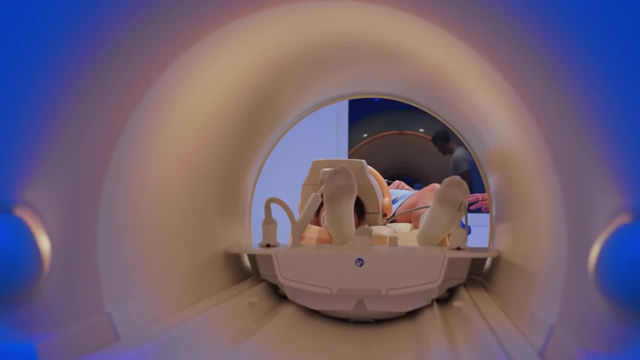 To avoid this refilling problem, modern MRI machines use a vacuum sealed chamber that holds the liquid helium without letting it evaporate. This eliminates the need for refilling and minimises the cost of operation. These so-called zero-boil-off machines are now the norm in MRI. 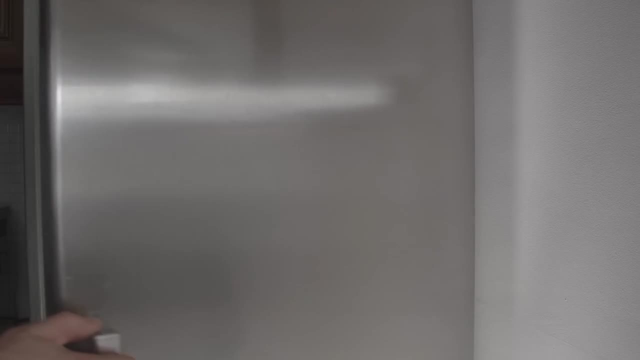 technology. This means that if you have a vacuum sealed chamber that holds the liquid helium, you don't have to worry about it. They use an electric refrigerant cycle like the one in your fridge, but on steroids. This cycle keeps the helium in its liquid phase. 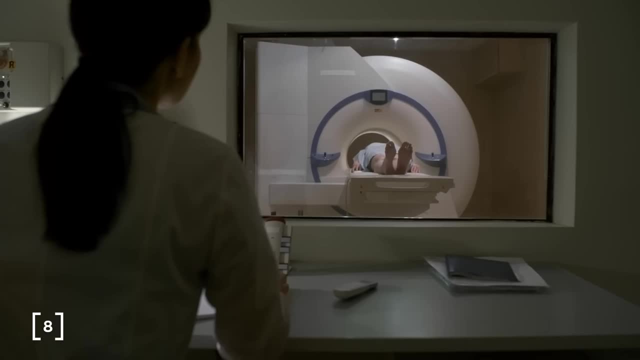 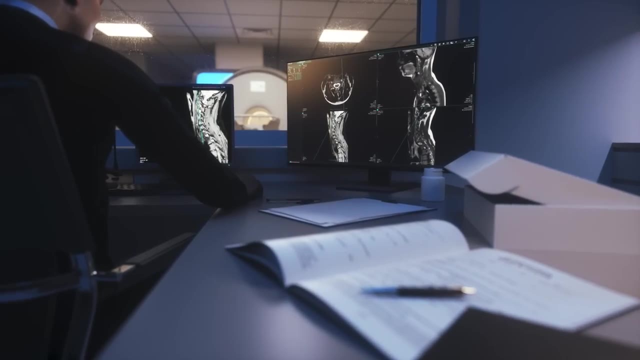 and keeps the magnets cool enough to maintain them in their superconducting state. Now that we know why and how the hydrogen atoms are aligned, we need a way to turn that information into an image, and to do that we need to know the physical location of the hydrogen. 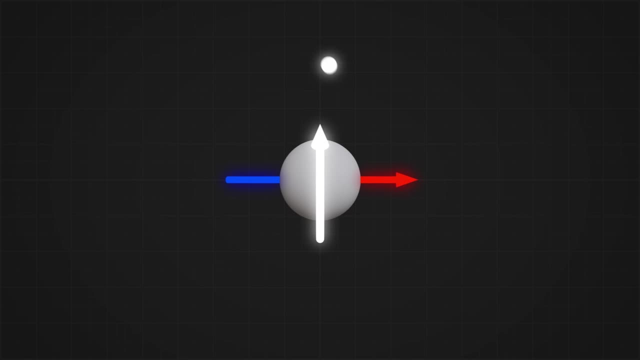 atoms Recall that MRIs detect signals from the spiral decay pattern of hydrogens. after the hydrogen atoms have been nudged, these spirals decay with a unique rotational frequency. Interestingly, this is the only frequency that can nudge the hydrogens too. 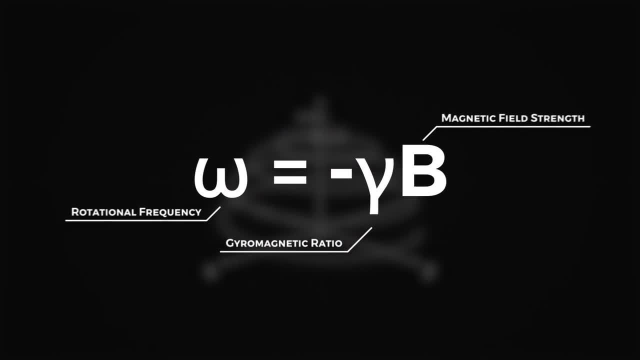 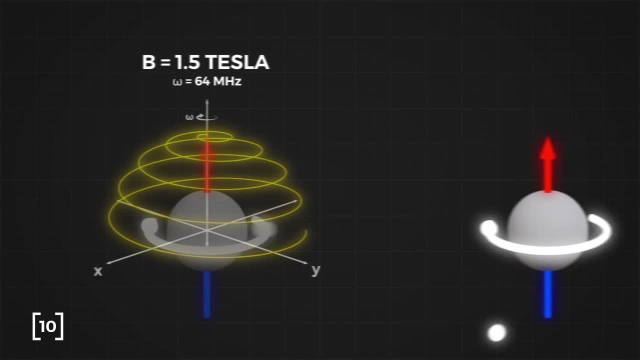 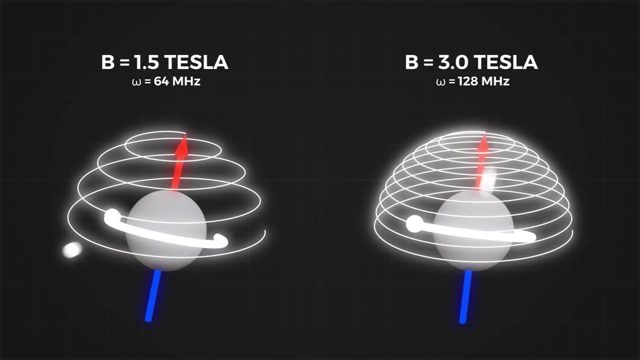 Luckily rotational frequency is dependent on something we control: the magnetic field strength. For example, hydrogen resonates at 64 megahertz at 1.5 tesla and at 128 megahertz at 3 tesla. This means the atoms in a weaker magnetic field will rotate slower, while atoms in a 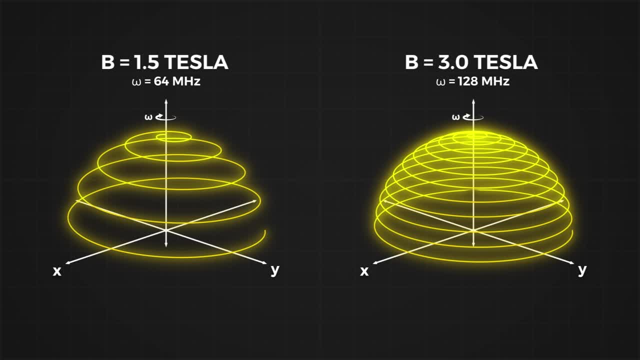 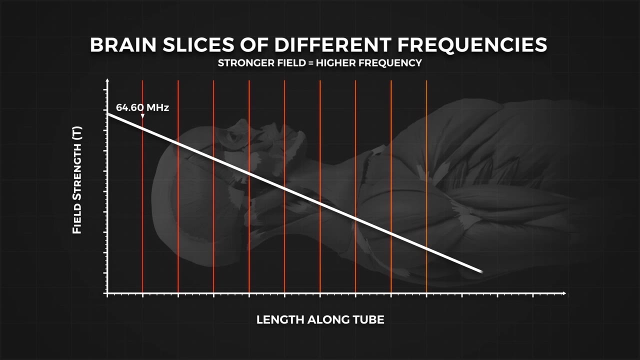 stronger magnetic field will rotate faster. To nudge these atoms we also need a radio frequency wave at 64 megahertz or 128 megahertz. We can use this to our advantage to image individual slices. If we apply a gradient to the magnetic field strength, we can selectively nudge atoms along. 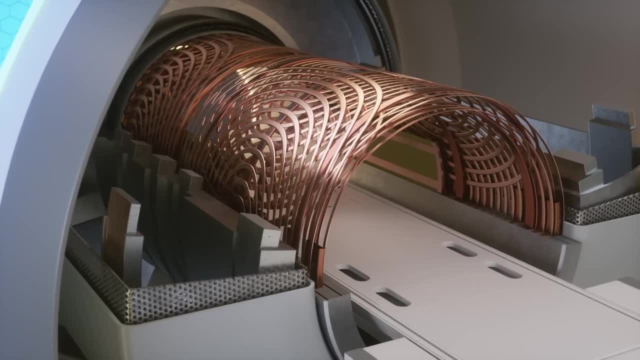 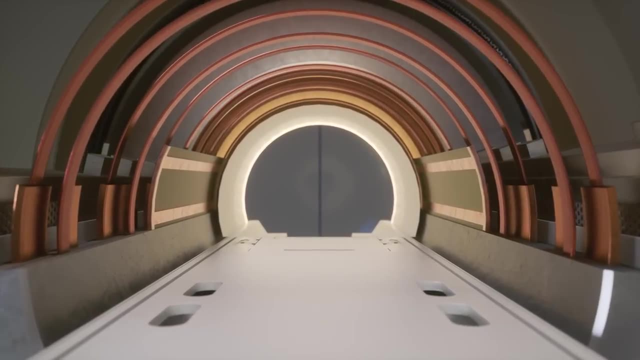 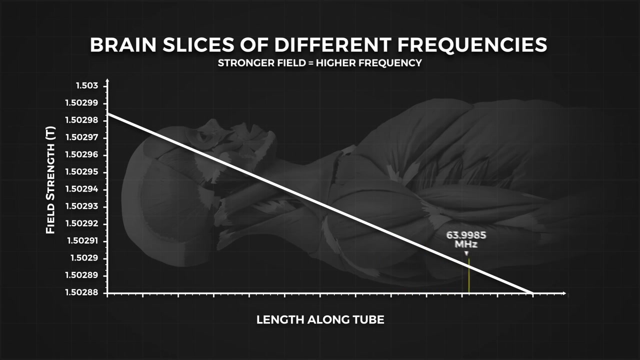 the gradient by applying the corresponding frequency. This gradient is applied precisely using a separate set of regular electromagnets, aptly named gradient coils. To image a slice near the weaker end of the tube, the machine sends a nudging pulse centred at the lower rotational frequency, say 63.998 megahertz, And to image a slice on the, 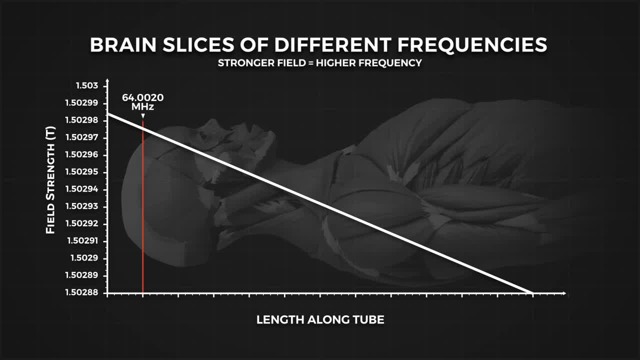 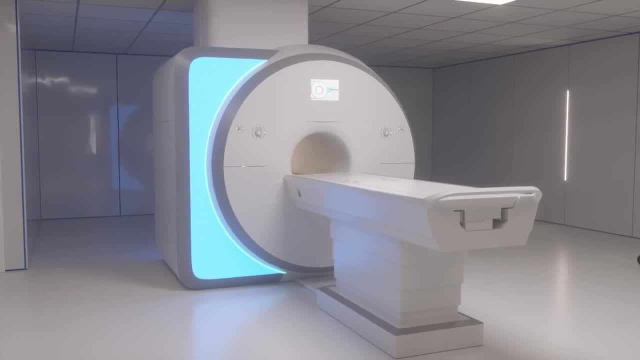 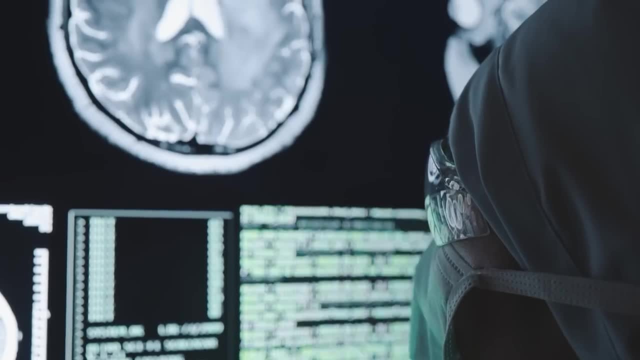 other end of the tube, the pulse is centred at 64.002 megahertz. This still feels like magic. It's not terribly obvious how detecting the decay from the spiralling hydrogen atoms can create images. The receiving coil can only measure the sum of all of the spiralling decays. We need a way of processing the signal to create. 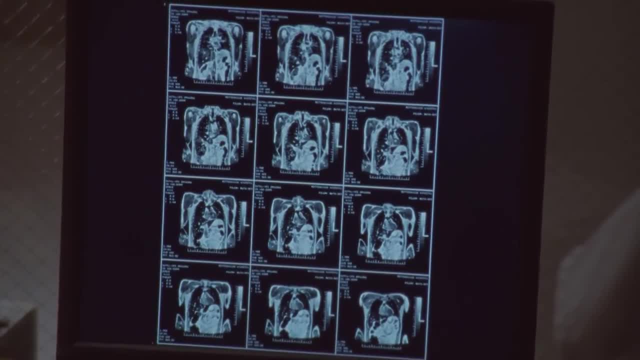 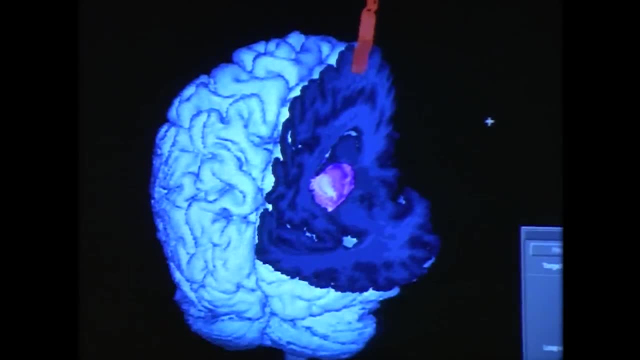 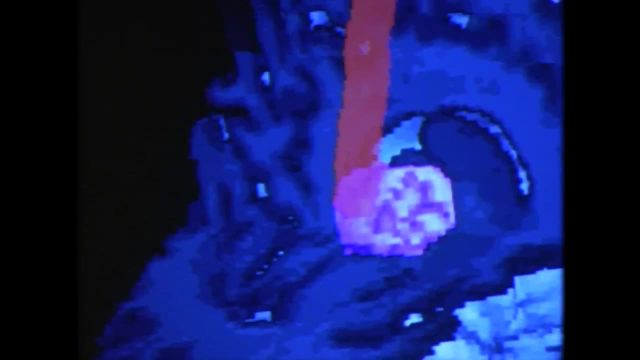 an image. Let's start by understanding how to get contrast between tissues before delving deeper into the technologies used to actually form images. We need a way of identifying different kinds of tissues to form an image. To do that, we need to contrast the tissues using two different 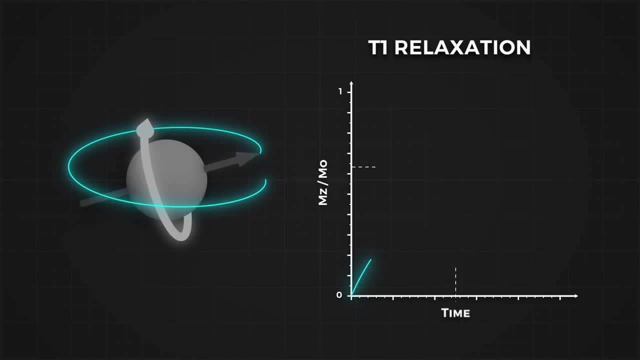 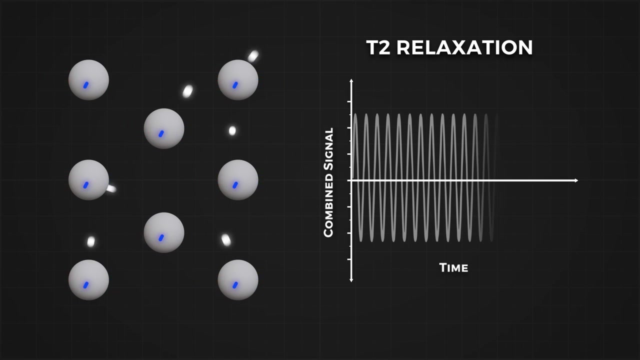 signal types. The first one deals with how quickly atoms realign themselves with the large magnetic field after a nudging pulse. This is called T1 relaxation. The second measure comes from the physical reality of interaction between hydrogens. The atoms do not realign with the magnetic field uniformly. In tissue, hydrogens interact with each. 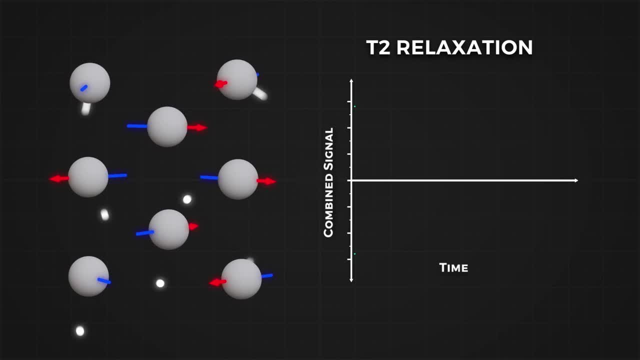 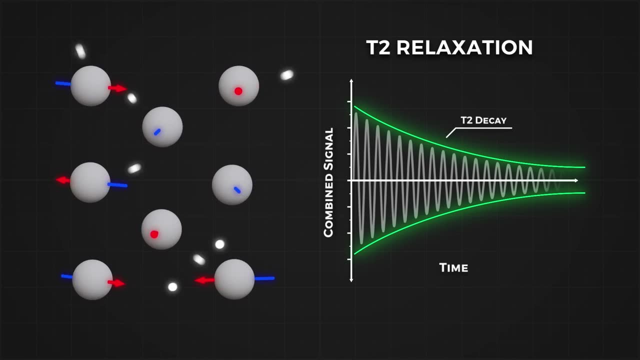 other and with their surroundings. Right after the nudging pulse is sent, the small interactions cause the spins to fall out of uniformity. Since the coil can only measure the sum of all of these spiral decays, then the falling out of order would create a decaying signal. 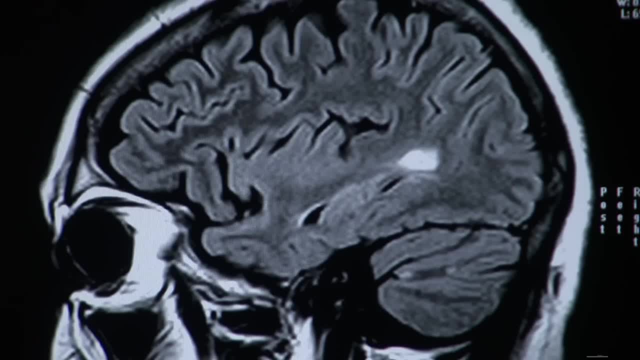 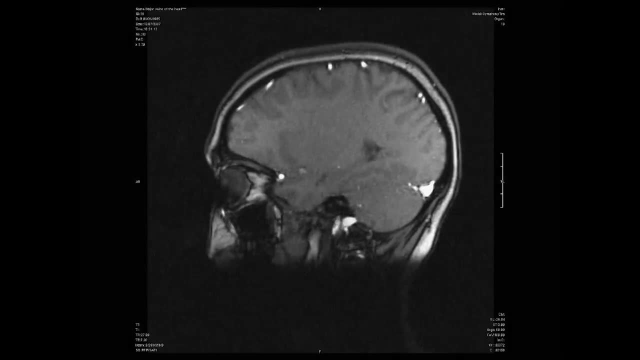 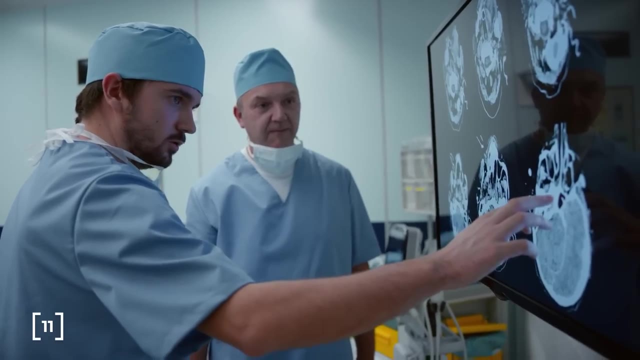 This is called T2 decay. Importantly, the two rates are not equal and, even more important, they are dependent on the tissue. Hydrogens in fat have different intrinsic characteristics and interactions than hydrogens in water. This difference is what lets technicians contrast the. 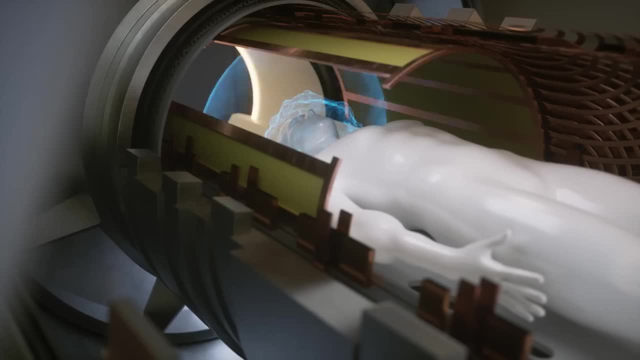 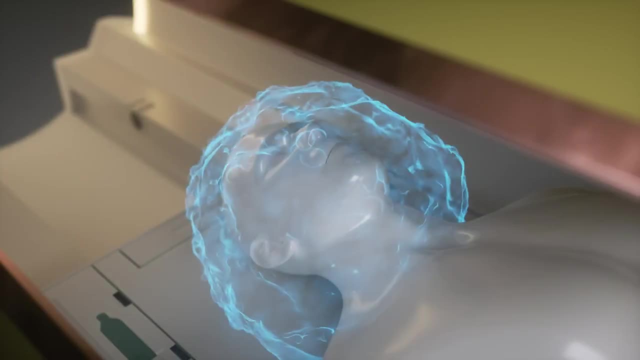 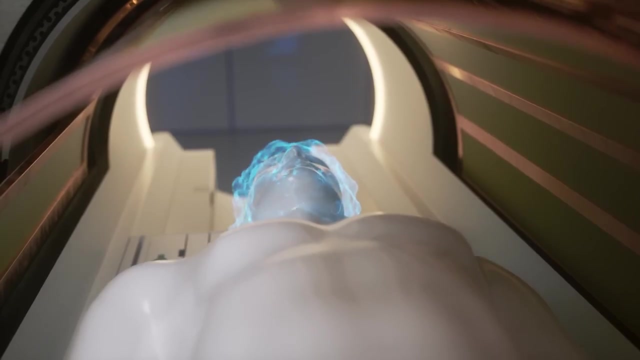 tissues. We can emphasize the T1 signal by sending pulses rapidly and listening to the signal immediately, as the dephasing effects of T2 do not have enough time to take place. We can emphasize T2 by sending pulses slowly and listening for longer, allowing the dephasing to. 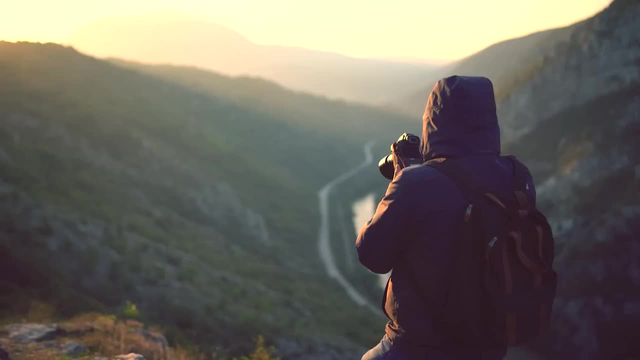 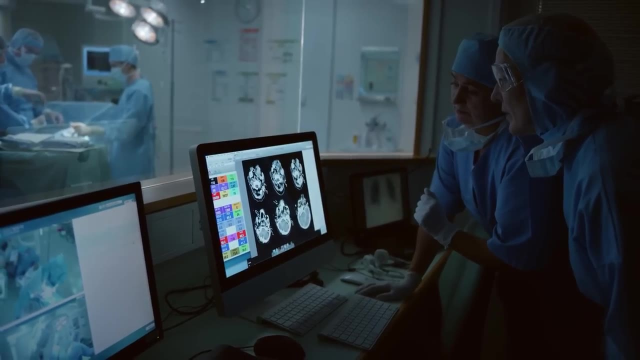 occur. Just like a photographer can play with camera settings to take pictures of either the bright sky or a dim environment, MRI technicians can also play with two settings to take images of contrasting tissues, The time between pulse repetition and how long to wait to listen for. 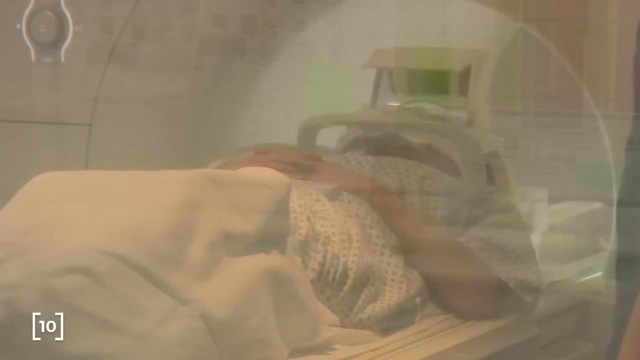 a signal. The second measure comes from the physical reality of interaction between hydrogens and water. These two parameters are chosen by the technician each time an MRI is performed, and they choose them depending on what the doctor would like to image, For example. 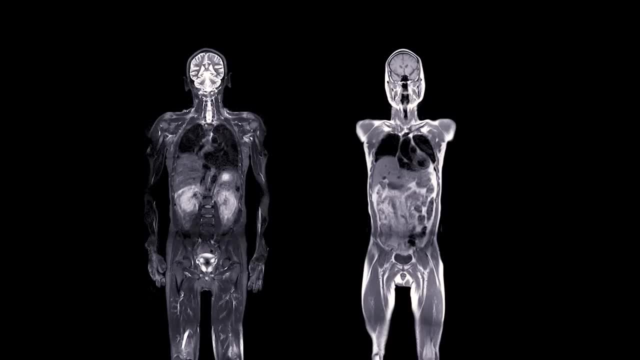 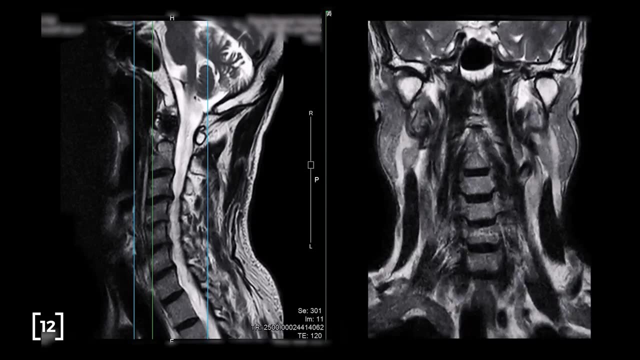 T1 is used to image fatty tissues while suppressing the signal from water. But maybe the doctor wants to assess the cerebral spinal fluid in the spine or the brain and for that T2 signals are emphasized to enhance the signal from water based fluids. 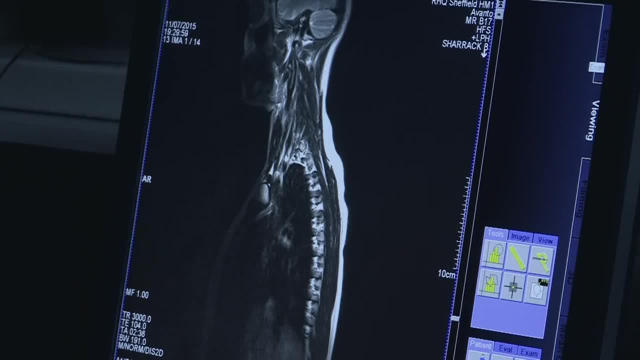 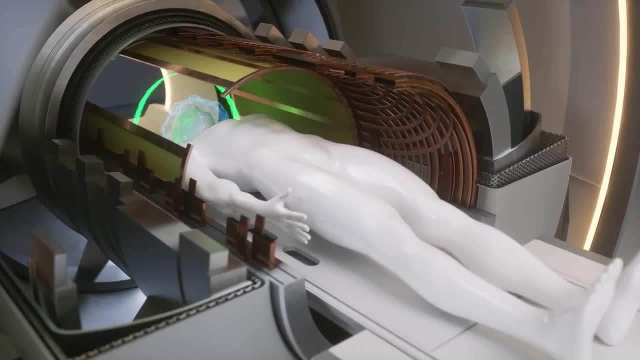 Remember, the signal is collected as a sum from a singular slice. The machine needs to form a 2D image of each slice. There is one extra layer of complexity since the receiver coil can only measure the sum of the signals from all the decaying hydrogens. 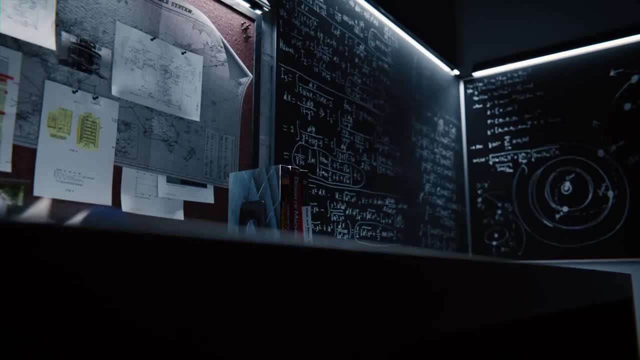 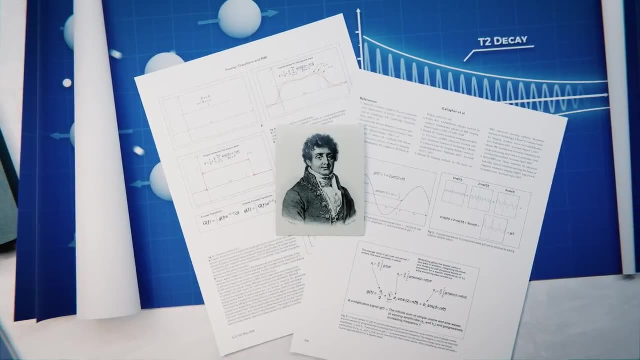 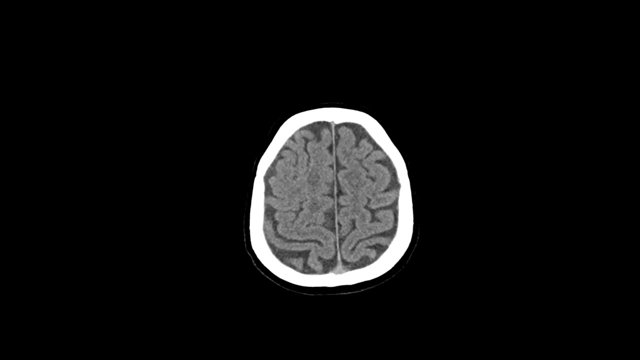 in the slice. This is yet another story where old mathematic discoveries guide modern technology. In 1822, Joseph Fourier created a mathematical framework that deconstructs complex waves into simple additions of simpler waves. This framework can be extended to 2D greyscale geometries, just like a musical melody can be simplified. 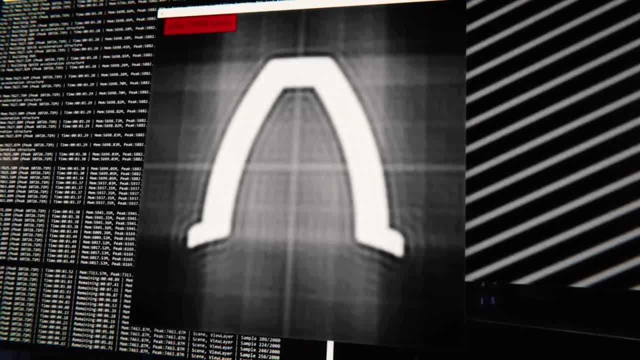 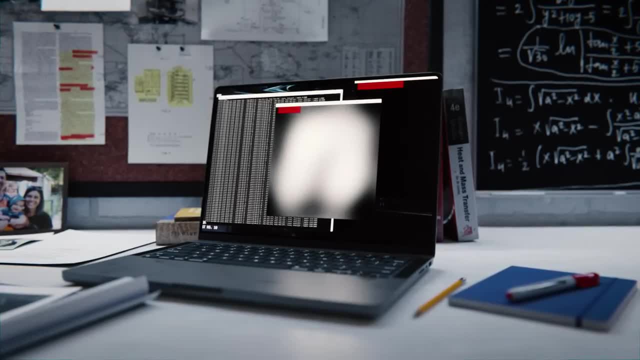 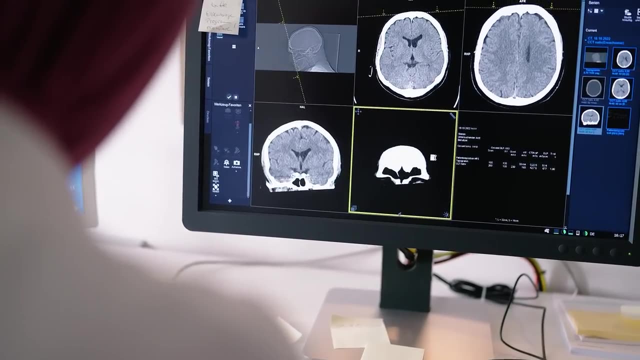 into additions of simpler notes. Any image can be deconstructed into a weighted average of simpler black and white stripes. This is what MRIs use to create images. Instead of sampling individual pixels, MRIs sample different striped patterns In reality. what does this mean for the spinning? 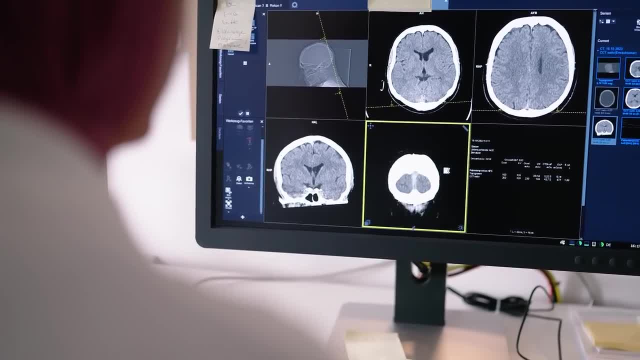 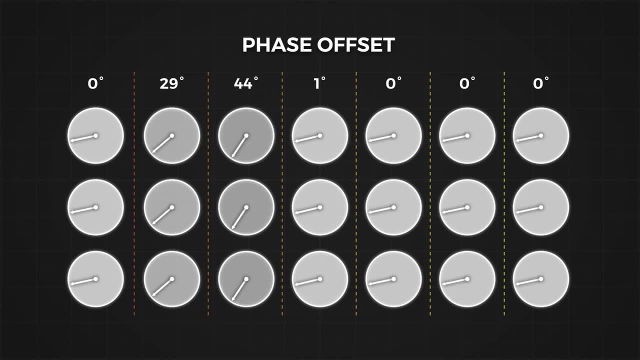 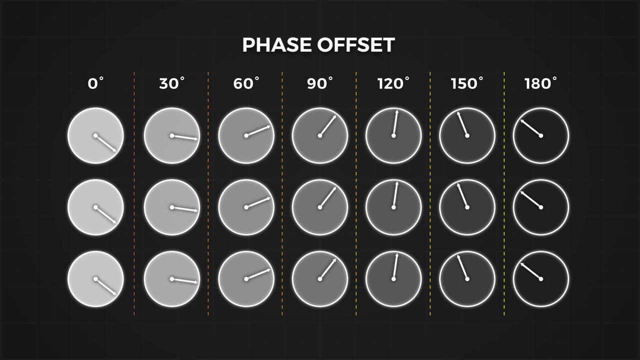 hydrogens. What is the physical representation of these patterns? It is easier if we imagine the slice as a grid of rotating hydrogens where we colour the phase of the atoms in greyscale. When rotating in unison, the grid is all white and atoms rotating 180 degrees out of phase are. 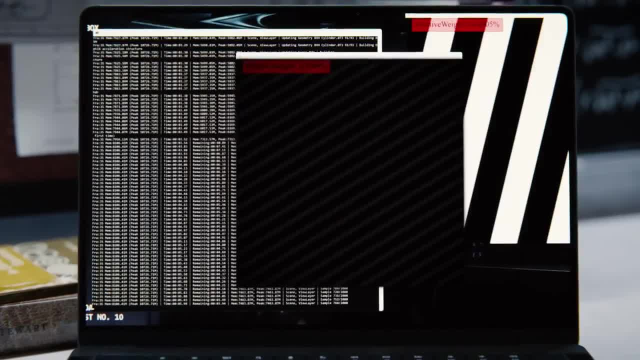 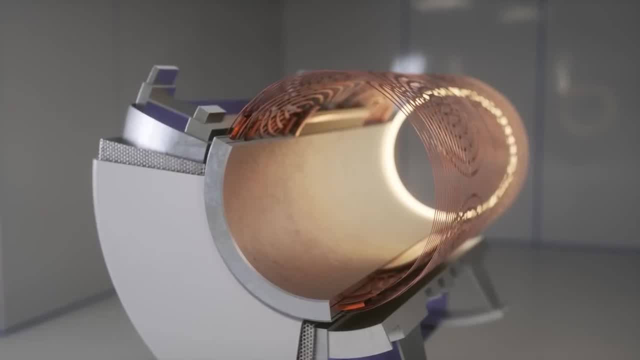 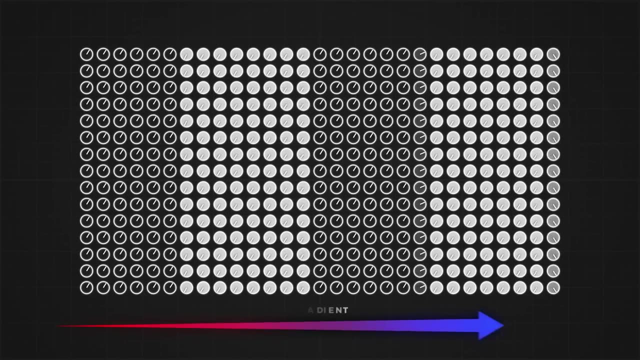 coloured black MRIs exploit this to physically create the striped patterns needed for the Fourier analysis. Using another set of gradient coils, MRIs precisely change the phase of rotating hydrogens to create striped patterns By controlling how long the y and x gradients are turned on. the MRIs can create patterns in all directions and frequencies Slowly. 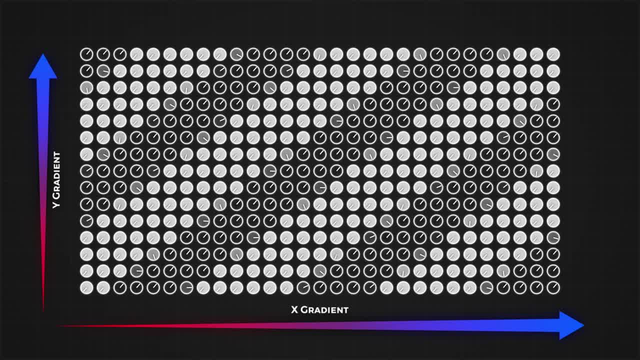 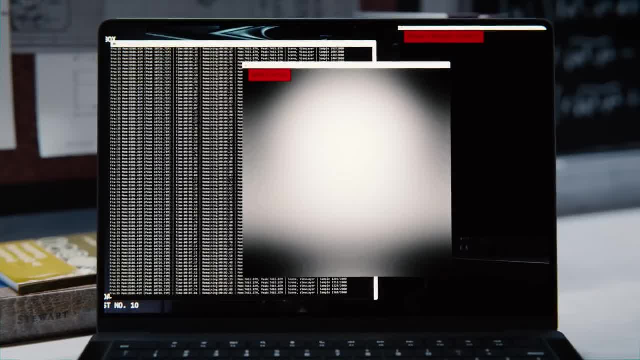 the machine starts to imprint all the patterns with different frequencies and orientations to sample their relative strengths in physical space And slowly, by adding more and more patterns, the image starts to emerge. This is what forms the image for each 2D slice. 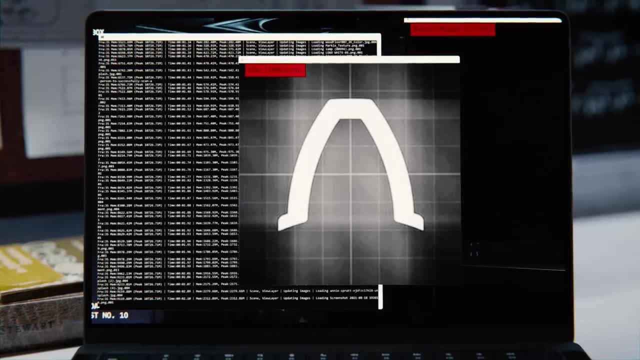 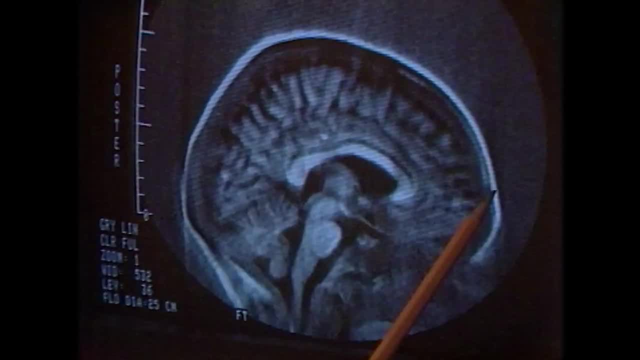 Then the machine goes on to the next slide. Then the machine goes on to the next slide And starts the process all over again, Turning on and off the coils inside a magnetic field might sound familiar if you've ever played with a speaker. They are basically doing the same thing: Gradient coils, rapidly turning on and off. 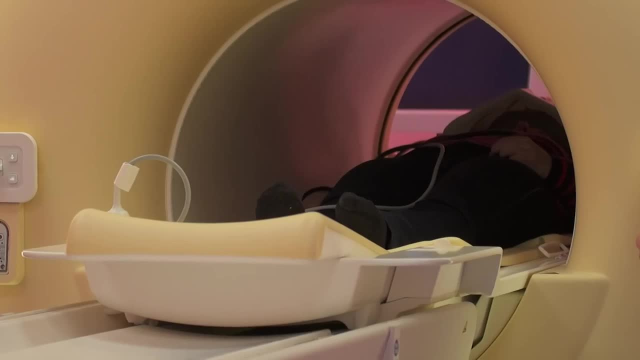 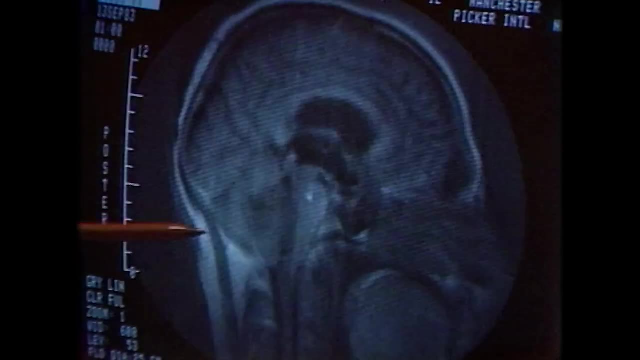 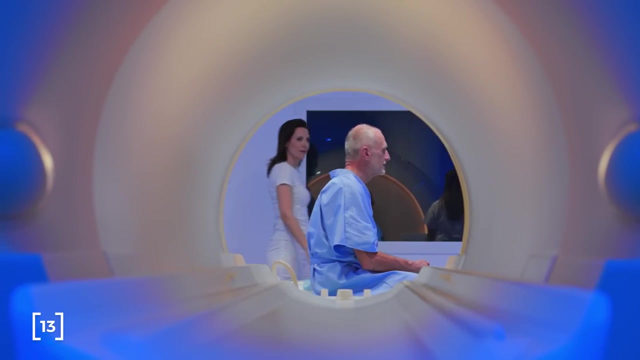 are the source of the loud clunking sounds in MRIs. MRIs are constantly evolving and the core technology is starting to branch off. Researchers want the highest resolution and strive to increase the strength of the magnets, while some hospitals and companies are making them smaller and cheaper, as more practical and 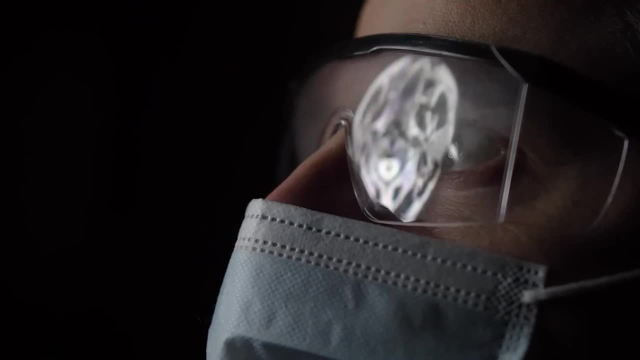 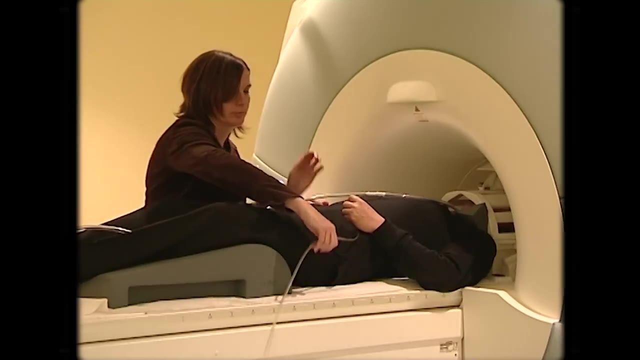 cheap MRIs are incredibly useful in the field. It's hard to fathom the complexity of all these systems, from superconducting wires to vacuum sealed helium reserves, to rapidly changing magnetic gradients. And it's even more incredible to think of the first people who figured out how. 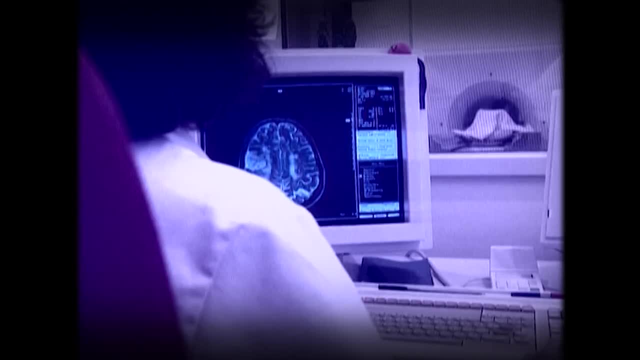 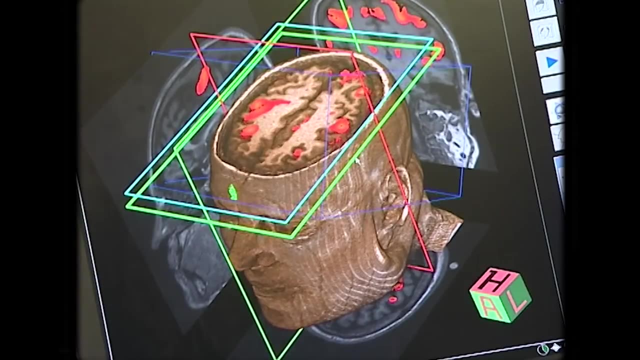 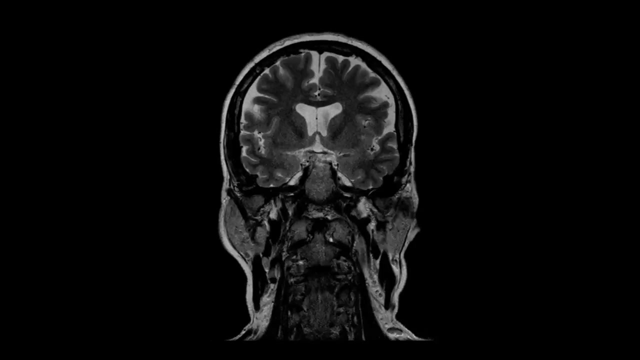 to combine these technologies together to peer into our bodies. This intricate dance of quantum physics and carefully manipulated gradients are now the real challenge of our times. This is an gradients has allowed MRIs to change the world of medicine. The MRI machine is a truly astounding piece of electronic technology and developing something. 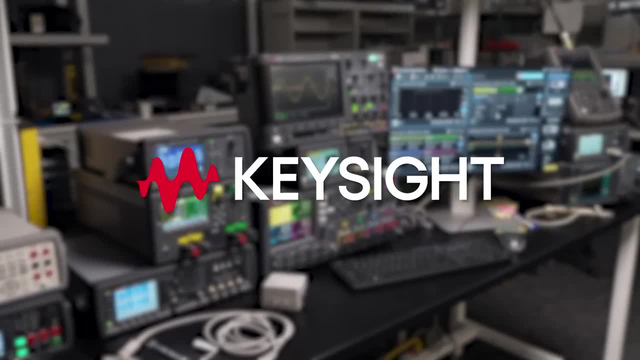 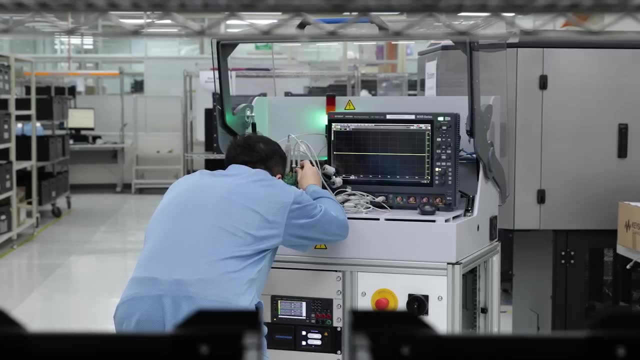 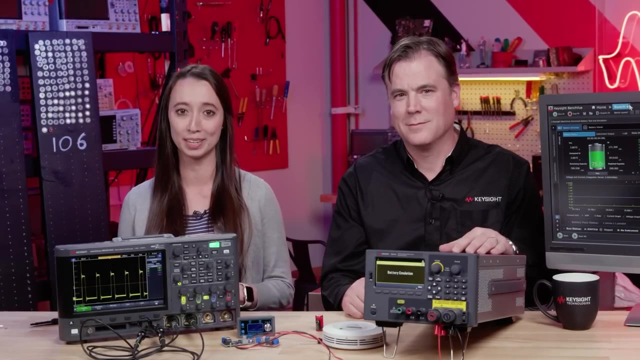 this complicated would simply not be possible without diagnostic tools like those created by Keysight. Keysight put the very best electronic measurement and testing tools into engineers hands and are holding another virtual event for engineers on May 16th. This fantastic free event is a rare opportunity to learn about electronics from experts. 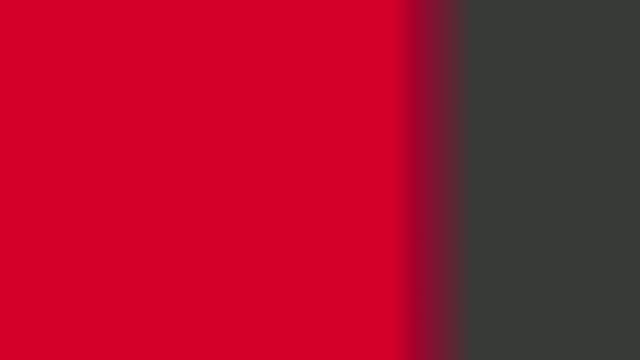 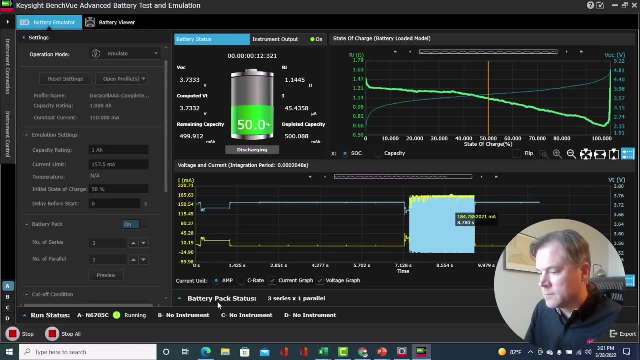 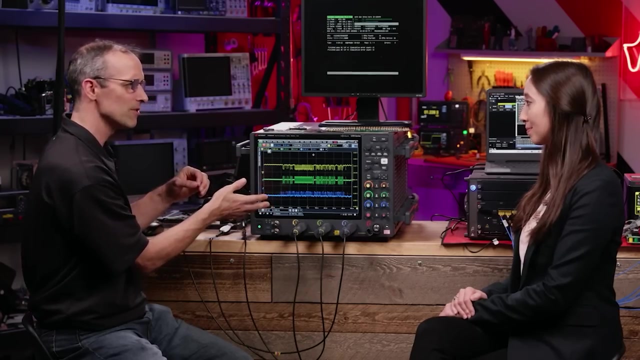 This event will explore performance of batteries, DC to DC conversions and internet of things devices, using live experiments like testing different battery models at different temperatures to see how that affects device runtimes, and testing DC to DC converter performances. This isn't just a live video you can watch and learn from. there will be a live Q&A session. 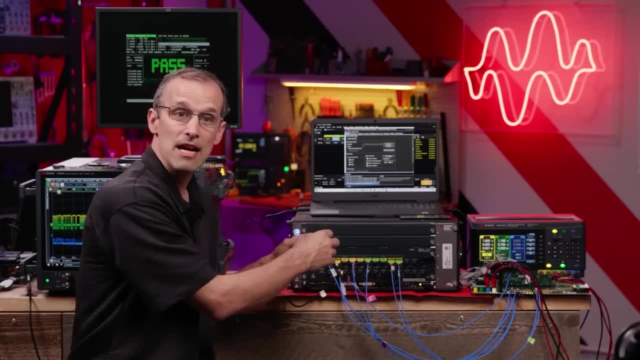 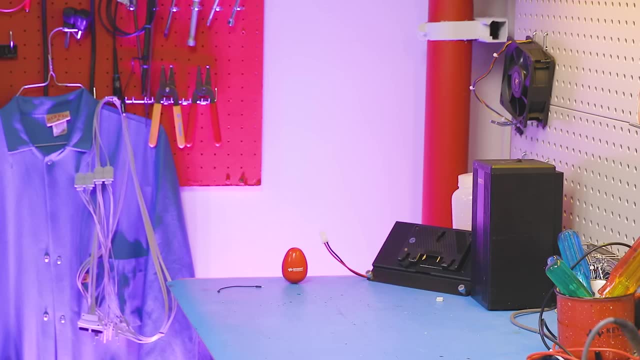 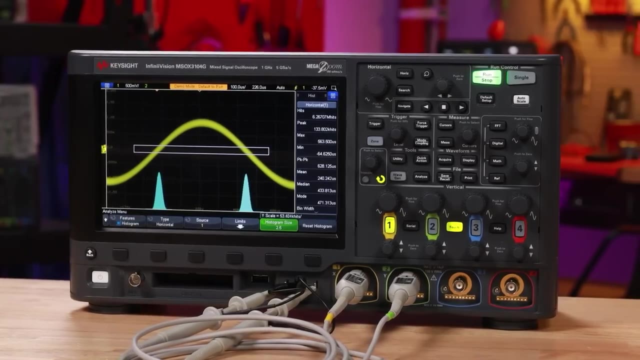 too, Allowing you to ask industry experts questions, An opportunity that does not come around very often- and everyone that registers for the event will be entered into a draw for Keysight's massive gear giveaway. They are giving away 20 pieces of pro grade test gear worth over $300,000. 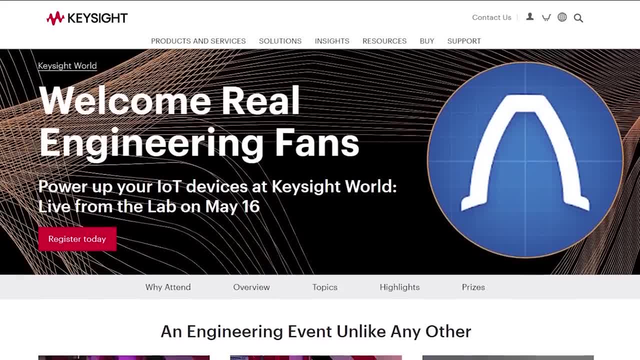 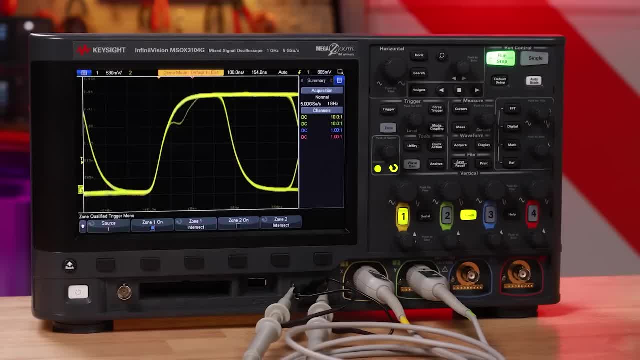 These are extremely valuable professional grade tools and you will get an extra entry to the giveaway if you sign up with my link. If you missed this event, don't worry, because you can rewatch the stream and they will be holding new live events every two months. 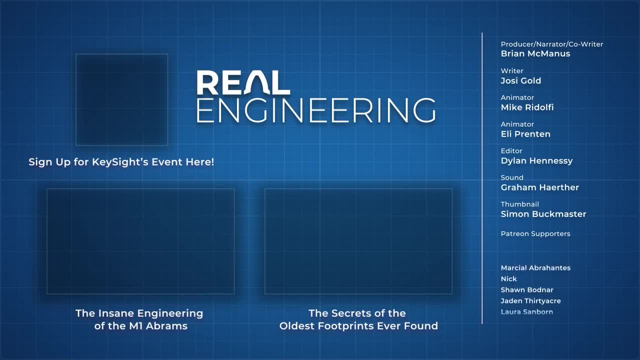 Whether you're an expert engineer or electronics newbie, you should definitely be signing up for this completely free event.